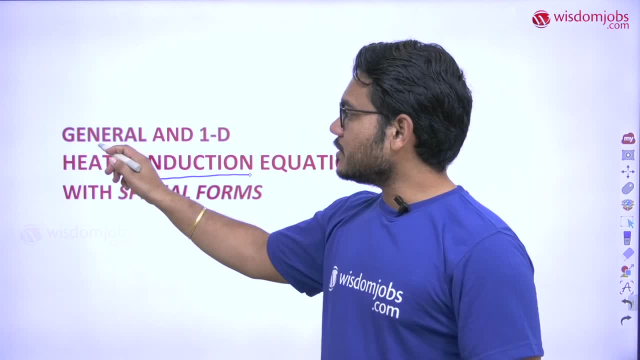 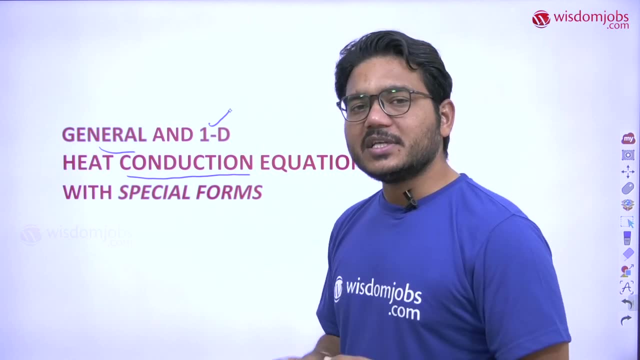 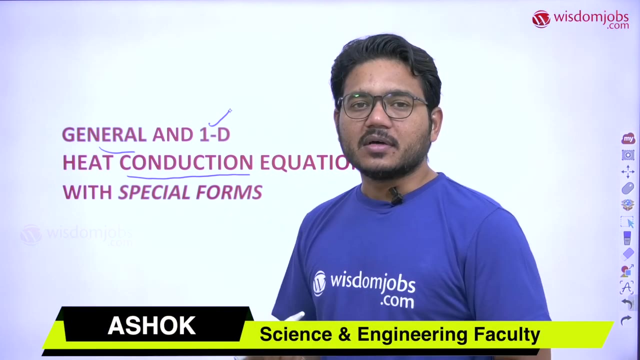 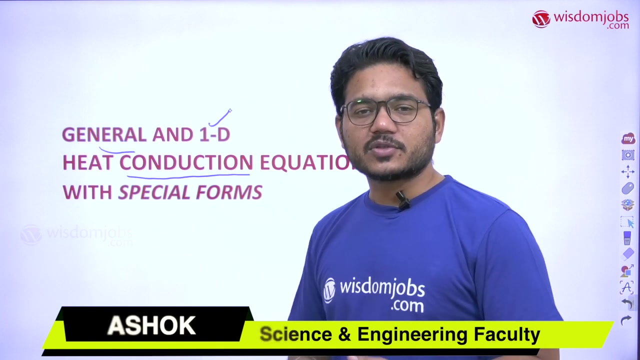 This conduction we will be studying So that general form we will be seeing initially The electron. we will be seeing one dimensional Because most of the applications, it will be easy to simplify it to one dimensional and study. Okay, Although in general cases not upon approximation, in generally in all the three directions, all the three spatial directions. so we have the change in means heat will be transferred. 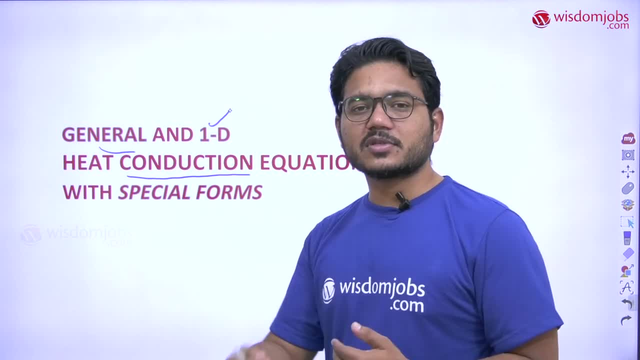 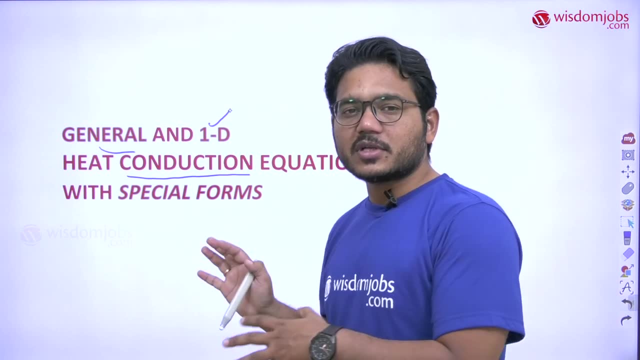 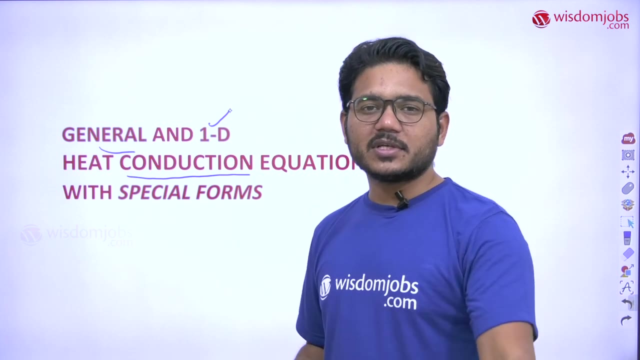 Okay, But sometimes based on the problem, based on the requirement, so we will be approximating it to, we will reduce the dimensions. So most of the cases in this particular engineering, heat transfer, studying, your BTech courses are coming to this elementary level. I mean school level. 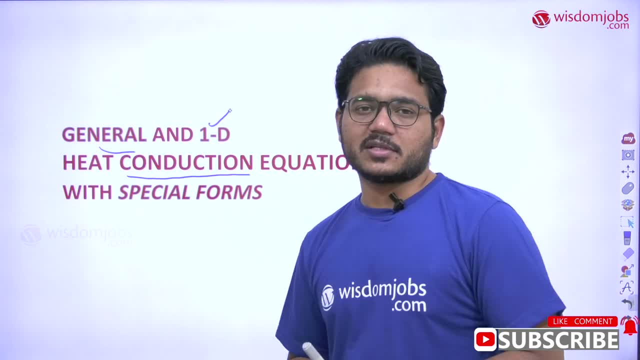 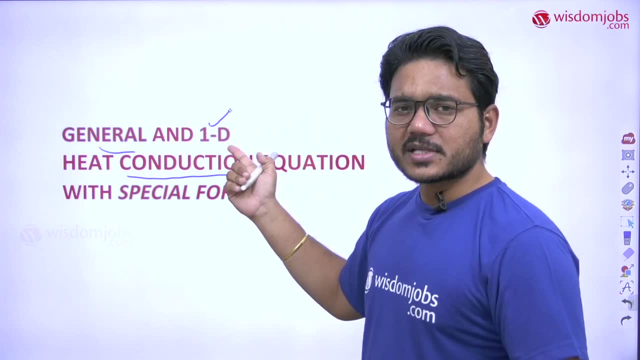 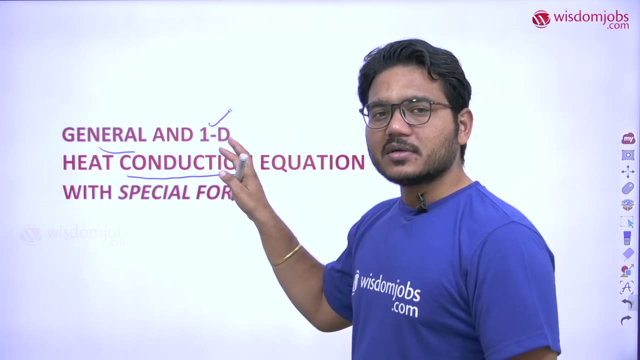 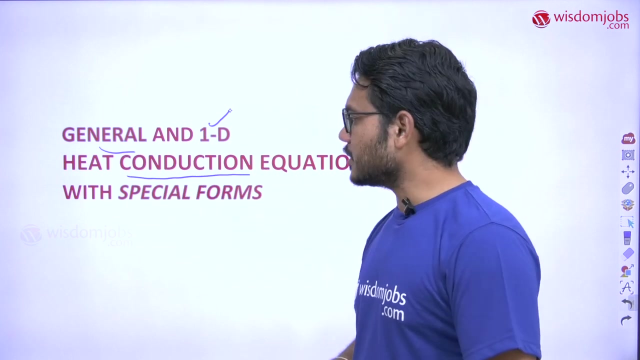 So you will be studying only this one dimensional thing, isn't it So? basic definitions you study at the school level anyway. So that thing we will be studying one dimensional, which is very important Because upon approximation, suitable approximation. so we will be using most of the cases, this one dimensional. That's why these two are very important: generalized thing and one dimensional thing. 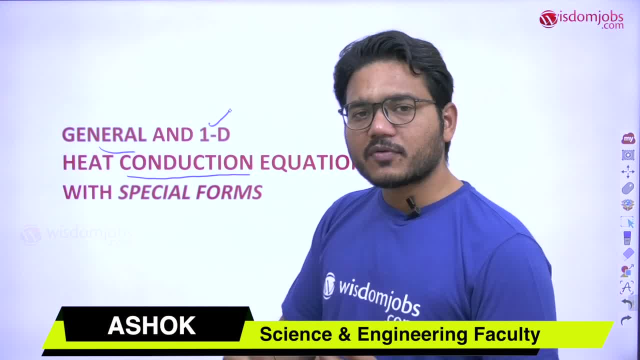 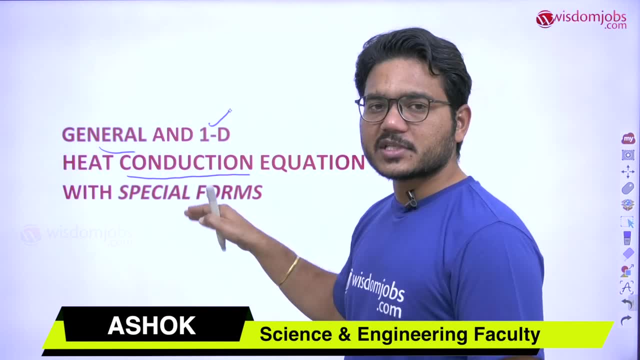 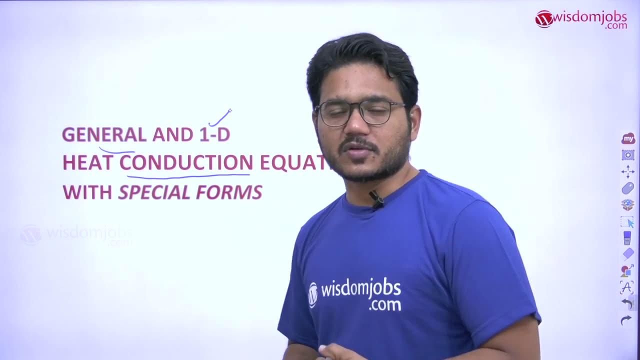